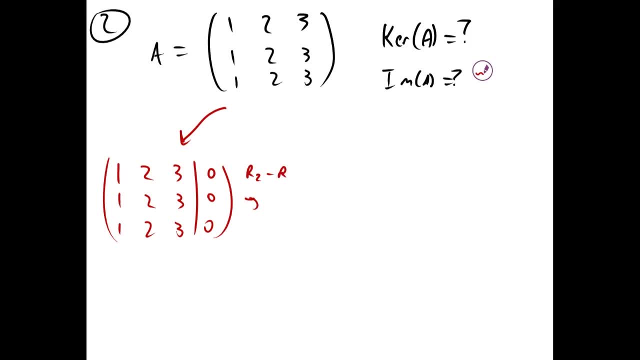 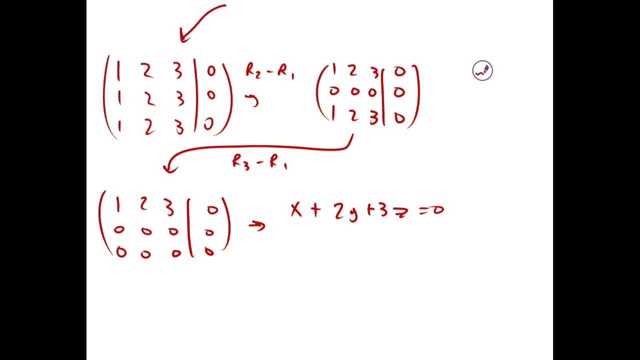 And if we subtract r2 by r1, and subtract r3 by r1,, we get 123 on top and then zeros for all the other entries, So now that we're in r3.. this tells us that x plus 2y plus 3z equals 0, y equals y and z equals z. 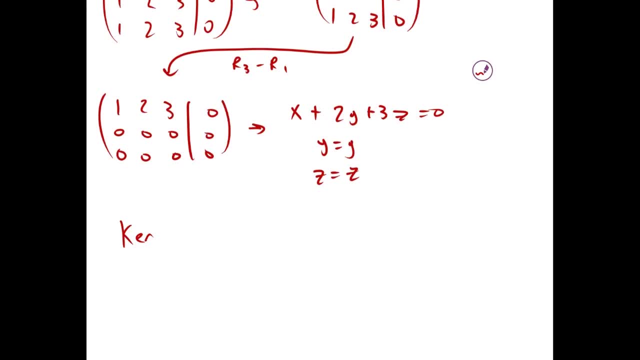 So the total of a is equals this set of x, y, z, that maps to 0, which equals minus 2y, minus 3z, y and z, which we can also write as negative 2, 1, 0 times y, plus negative 3, 0, 1 times z. 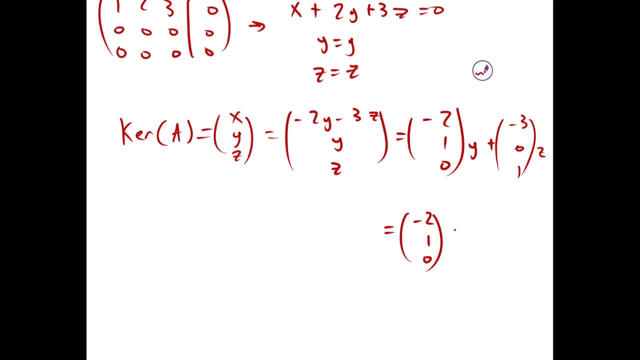 And we can just write those as parameters, t and s, With t and s coming from positive infinity to negative or negative infinity to positive infinity. So the kernel of a is the span of these two vectors, Span of negative 2, 1, 0, and negative 3, 0, 1.. 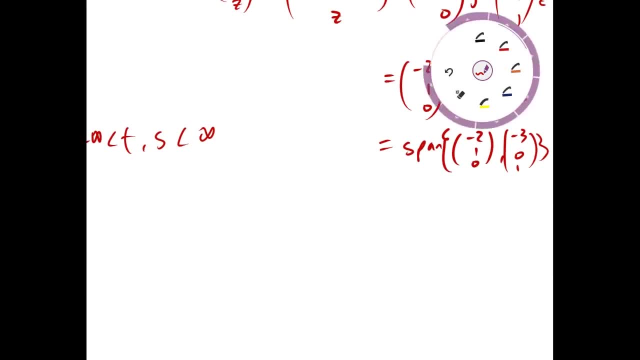 And we had to check for linear independence. but we can tell just by looking at it that these are because we have a 0. So we have a 0 here and a 1 here, then a 1 here and a 0 here. 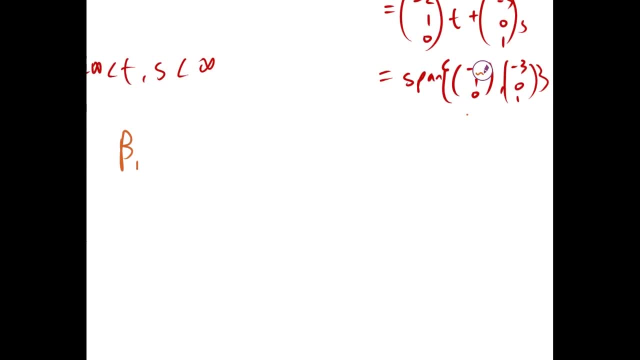 So if we wanted a basis for the kernel, we could just write negative 2, 1, 0, and negative 3, 0, 1.. So we omit the span. If we say span, we have an infinite amount of vectors. 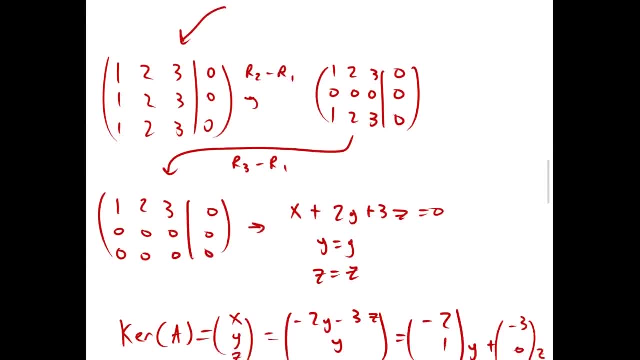 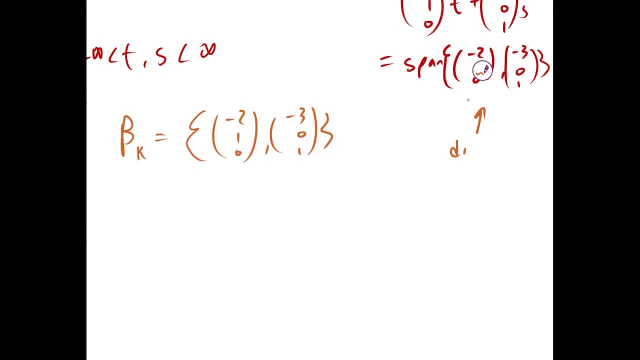 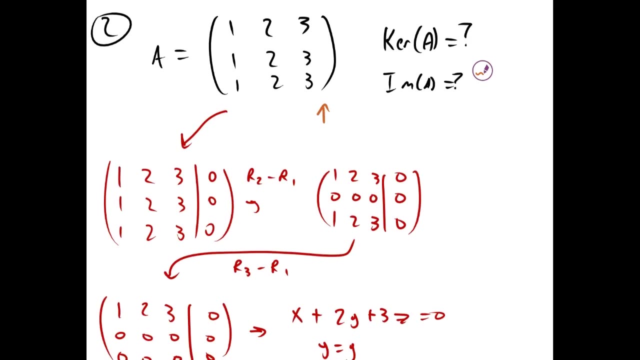 But if we just include these two, we have a basis So we can again check. we see that this has a dimension of 2, this kernel And by the rank, since we have an output of 3, because we have a 3 by 3 matrix, target space is 3,.